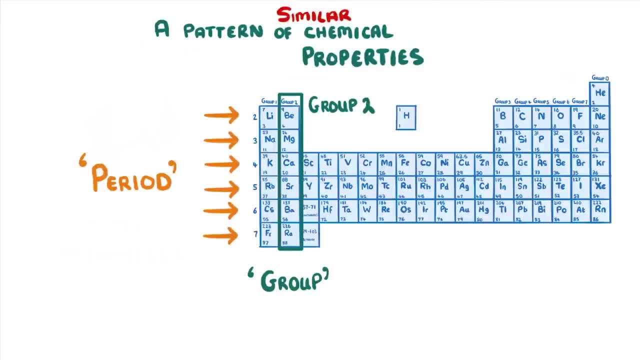 So here we're looking at group 2.. There are a couple of exceptions to this, though. One is that the far right group is called group 0, rather than group 8, and we'll take a closer look at why this is in a minute. 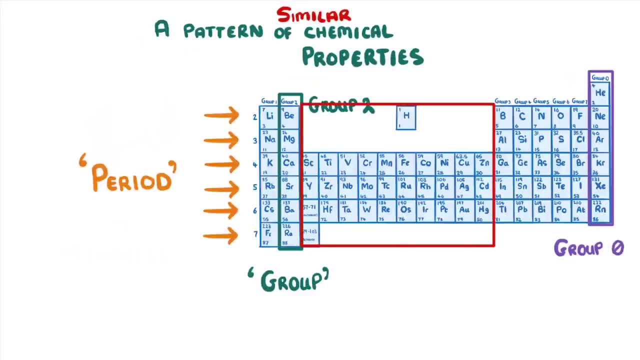 The other is that the block of metals between group 2 and 3 don't have group numbers. Don't worry about this for now, though. just remember to ignore them when counting your groups. The reason that elements in each group have similar chemical properties is that they 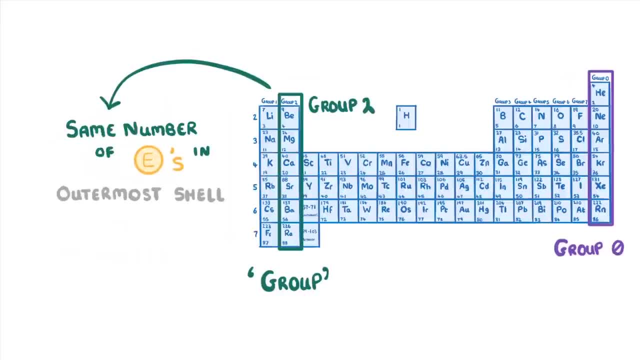 have the same number of electrons in their outermost shell, And this is largely what determines how an element reacts. In fact, the group number actually tells you exactly how many electrons they have in their outer shell. So as we're looking at group 2, we know that every element in this group has two electrons. 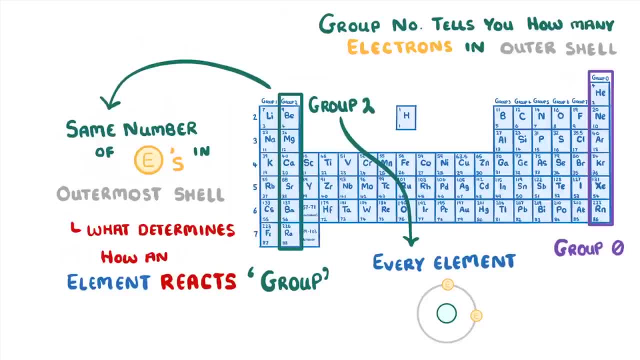 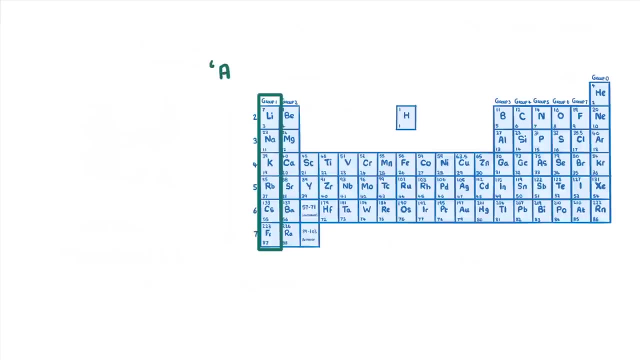 in its outermost shell. Just make sure you don't get confused here. All of the elements in a given group have different total numbers of electrons. they just have the same number of electrons in their outermost shell. So if we move over to the group 1, elements which we call alkali metals, we can tell. 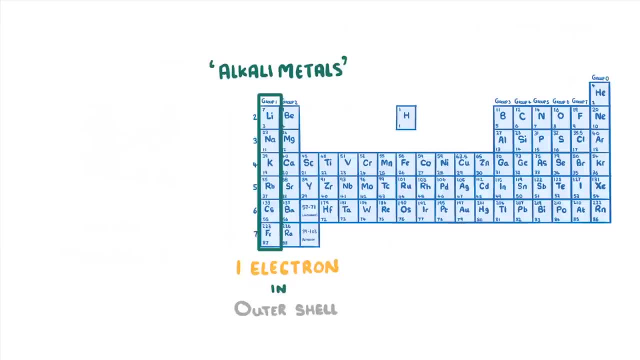 that they all have one electron in the outer shell, whether it's lithium, which has 3 electrons overall, or sodium, which has 11 electrons overall, And it's this feature that gives all group 1 elements similar properties. For example, they all react violently with water. 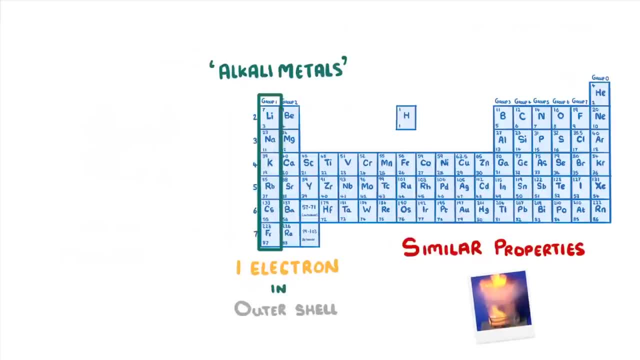 There are also trends within groups. For example, the group 1 elements become more reactive as time passes, As we'll see later in a video specifically on group 1 elements. Group 7 elements, meanwhile, which we call halogens, all have 7 electrons in their outer. 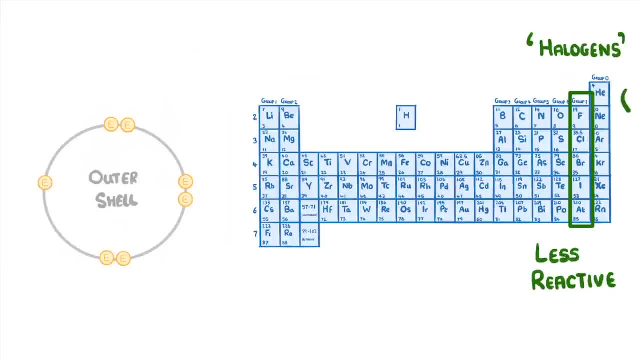 shell, Although these elements become less reactive as you go down the group. As we said before, group 0 is a bit different. These elements are called the noble gases and they all have full outer shells. So argon, which has 3 outer shells, has 4 outer shells. 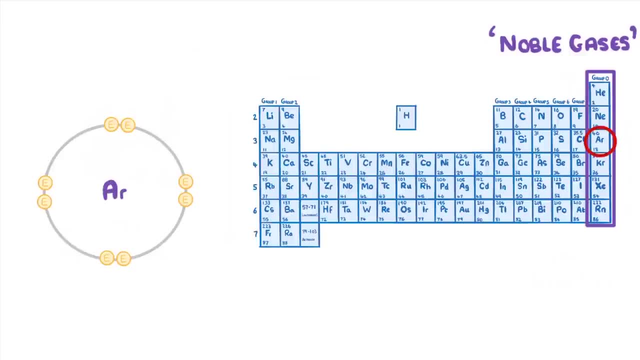 So argon, which has 3 outer shells, has 4 outer shells. So argon, which has 5 outer shells, has 6 outer shells. So argon, which has 0 out of 5, has 8 out of 8 in its outer shell. 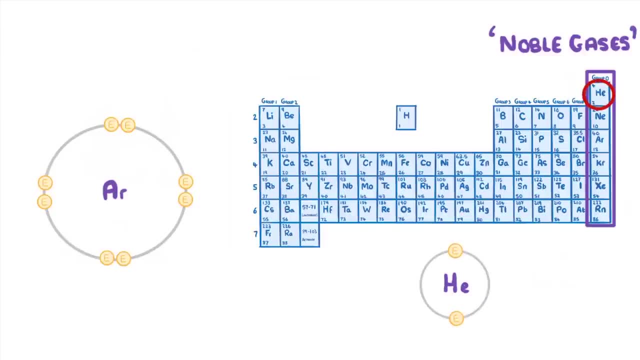 While helium, which only has 1 shell, has 2 out of 2. Because, if you remember, the first shell can only hold up to 2 electrons And because they don't need to gain or lose any electrons, the noble gases are all very. 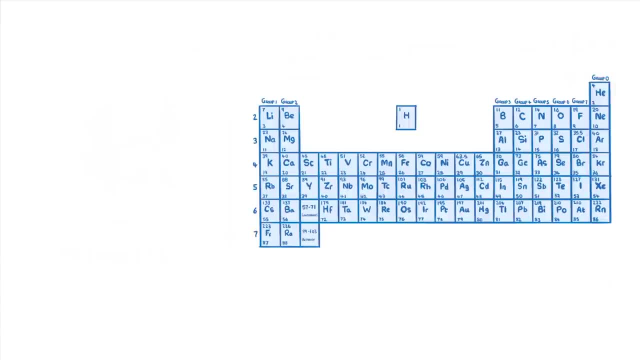 unreactive Number of electrons is as follows. Sometimes you might see a zig-zag line running here from aluminium to polonium. From them you can see 14 electrons. They're 2 under non-polymer metals, which include everything to the left in orange, from the non-metals on the right. 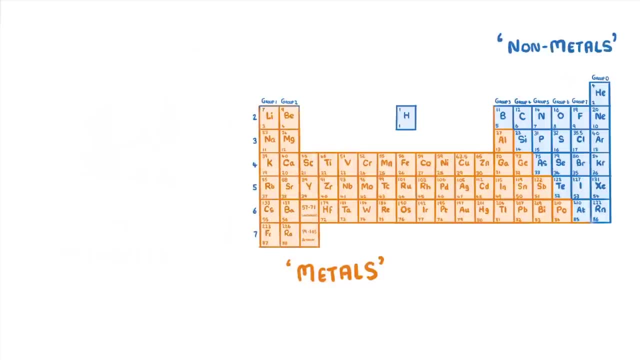 still in blue. So, as you can see, there are lots more metals than there are non-metals, And in the middle of the metals there's a special block of elements which are known as transition metals. We'll take a closer look at what these are in another video. just 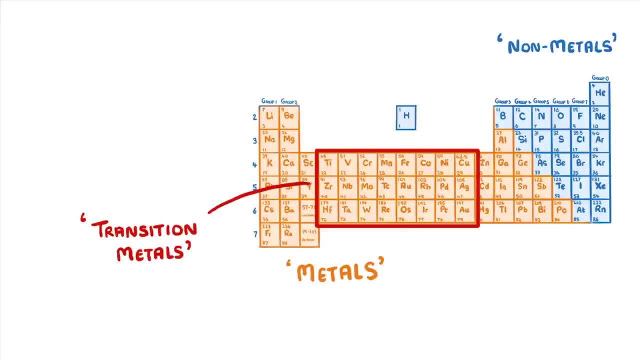 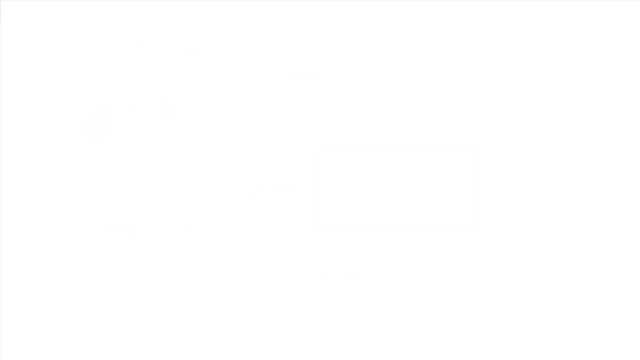 like. we'll take a closer look at the group 1, group 7 and group 0 elements and the differences between metals and non-metals. Before we finish, we just wanted to point out that if you google periodic table, you'll probably see loads of different types For. 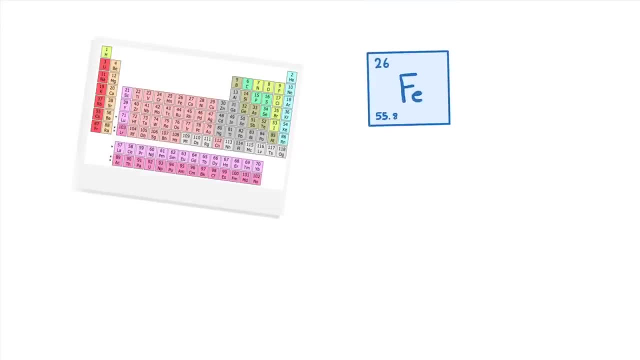 example, you might find that the position of the mass and atomic numbers has been reversed, like the example of iron here. Don't worry about any of this, though. the tables all show the same information, just presented in a slightly different way, And you can always. 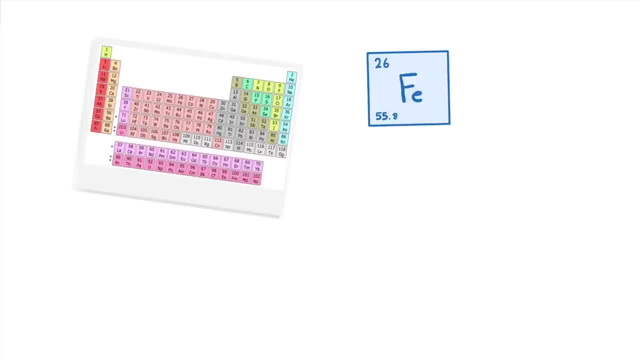 tell which is the atomic number because it will be the smaller of the two. And you can always tell which is the atomic number because it will be the smaller of the two. And in your exam, the periodic table you'll get given will be similar to the one we've. 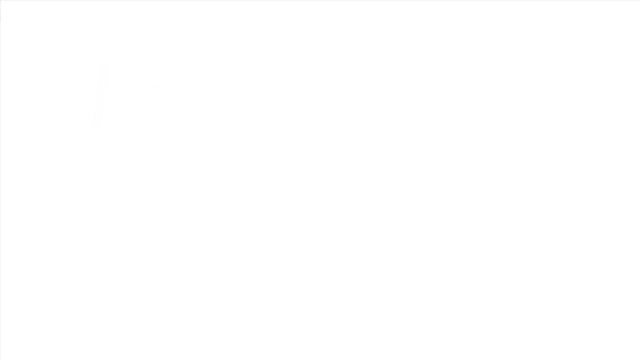 been using throughout the video. That's it for now, though. if you enjoyed it, then please give us a like and subscribe, and we'll see you next time. 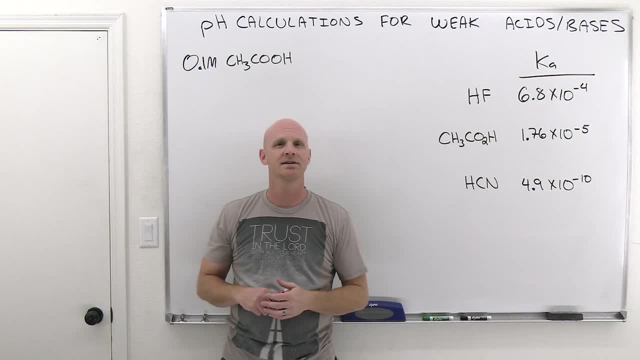 pH calculations for weak acids and bases is going to be the topic in this lesson. My name is Chad and welcome to Chad's Prep, where my goal is to take the stress out of learning science Now. in addition to high school and college science prep, we also do MCAT DAT.